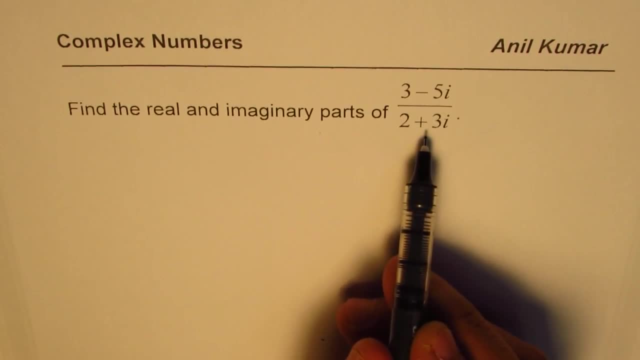 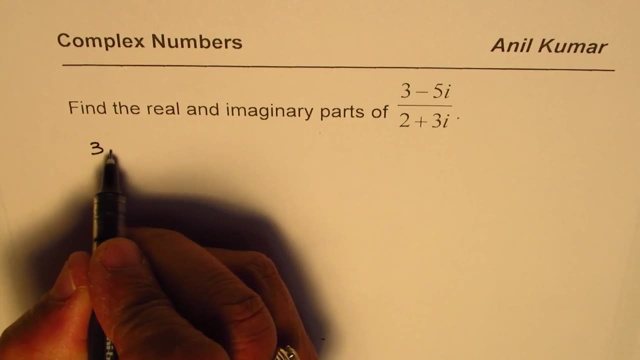 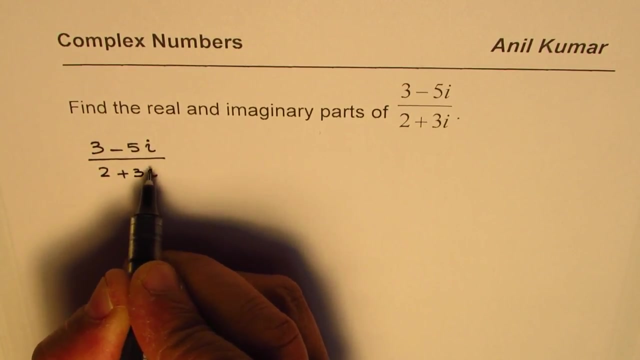 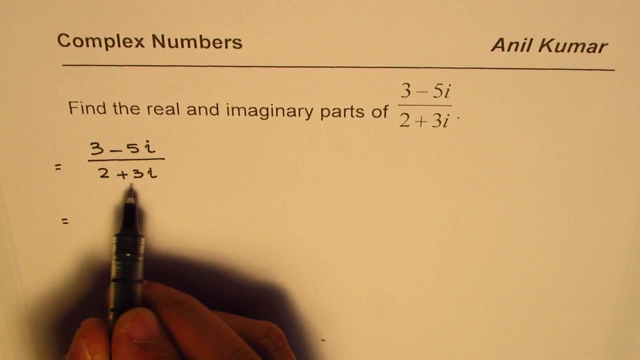 we should make the denominator real, and that process is called realization, right? So let's see how. So we are given complex number 3 minus 5i, divided by 2 plus 3i. Now if we multiply and divide this complex number by the conjugate of the denominator, then see what happens. 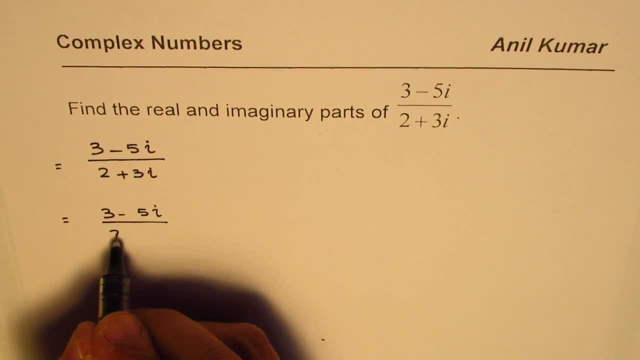 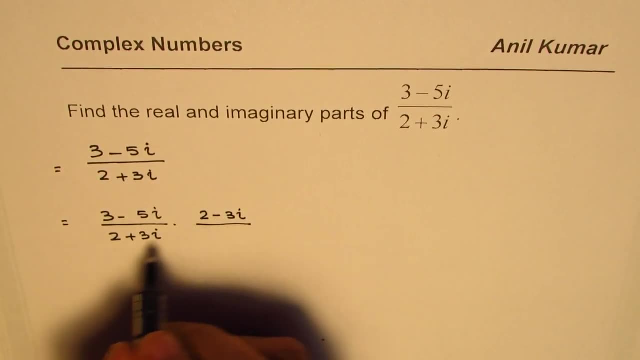 That is to say, we'll multiply and divide 2 plus 3i by 2 minus 3i. Now 2 minus 3i is conjugate of this denominator 2 plus 3i. So when you do so, denominator becomes 2 plus 3i times 2 minus 3i. that is 2 square. 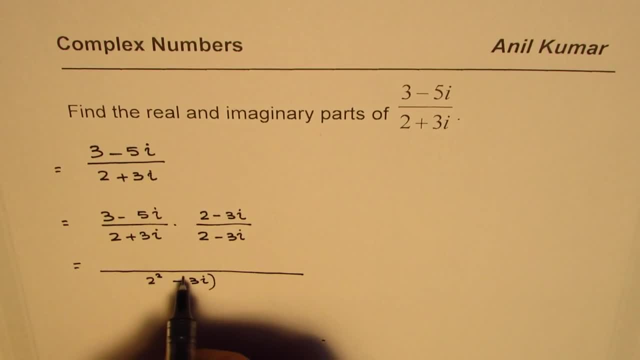 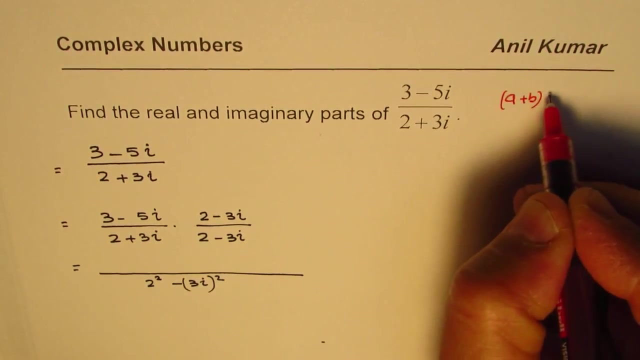 minus 3i square, right. You could expand using distributive property and then 2 times minus 3i and 3i times 2 will cancel out giving you this result right. Or you could use the formula, which is a plus b times a minus b is equal to a square minus b square Is: 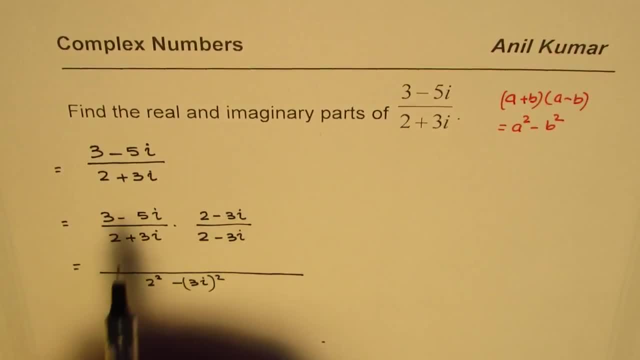 that correct. You could do it, or you could do distributive property, which we are going to do in the numerator. So 3 times 2 is 6.. 3 times minus 3i is minus 9i. Minus 5 times 2 is 10, and then i. 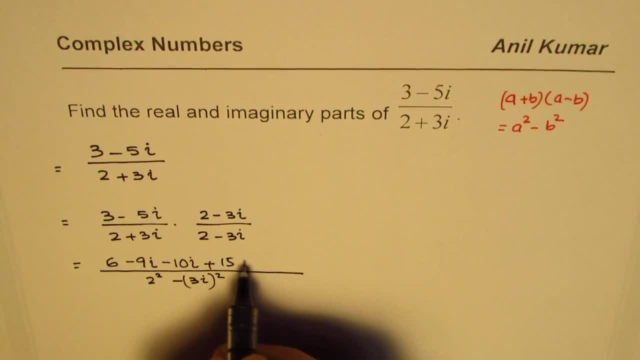 Minus minus becomes plus. 5 times 3 is 15.. i times i is i square, So that gives us 6 minus 9 and minus 10 minus 19, i i square is negative 1.. So we could write this as minus 15.. 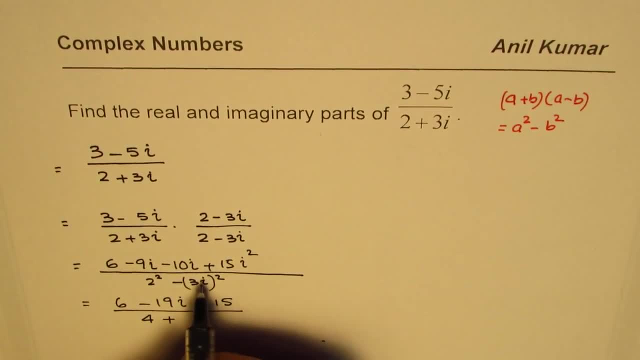 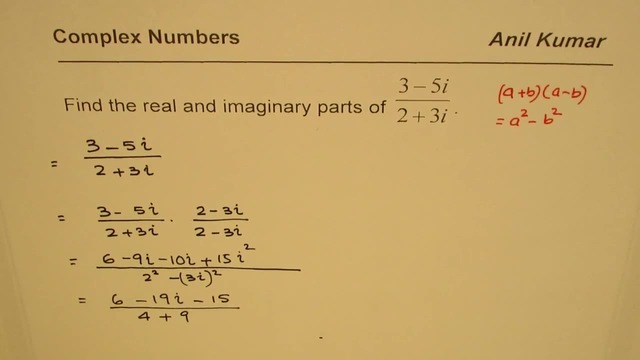 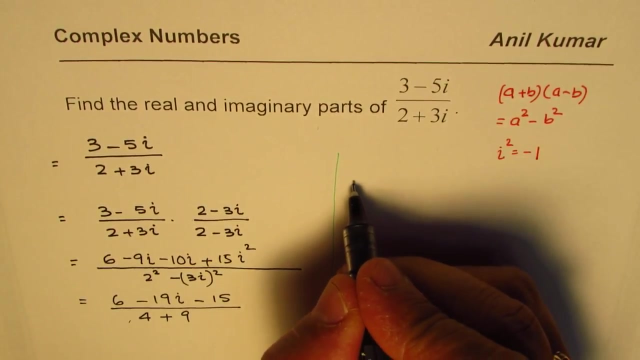 In the denominator we get 4 plus 3. square is 9. since i square is minus 1, the sign changes to plus right. so we know i square is equals to minus 1. so we have used that, so this sign becomes positive. now let's combine the terms in the denominator, so what we get, and also numerator 6 minus 15.